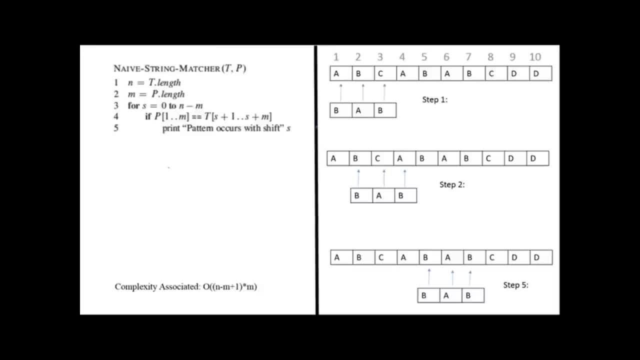 Text is always bigger in length as compared to the pattern And we will assign the length of the text to n and we will assign the length of the pattern to m: The length of the text to n and length of the pattern to m. Now, as we can see over here in the image, 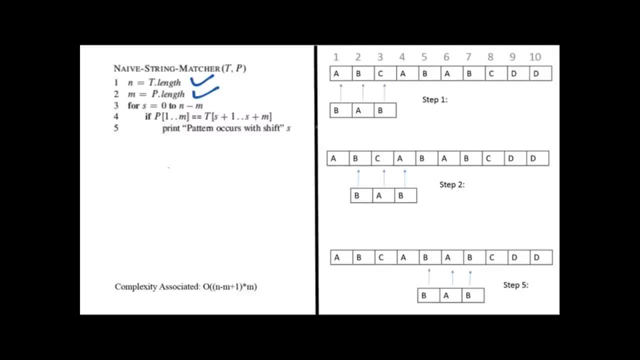 I will be basically correlating both the example and the algorithm together. So the pattern that we have over here is p And the text, as you can see over here, is of length 10, which is t. t is an array and the length of the text is equal to 10, as you can see. 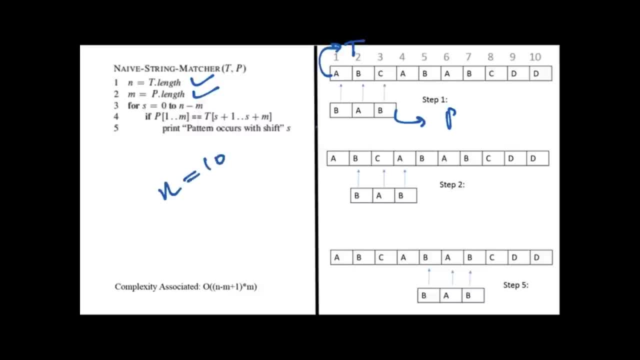 And we will assign this value to n. n is equal to 10.. Now we will be assigning the value m, equal to 3, as that of the length of p. Now we will start matching Here in the pattern. we have: b, a, b. 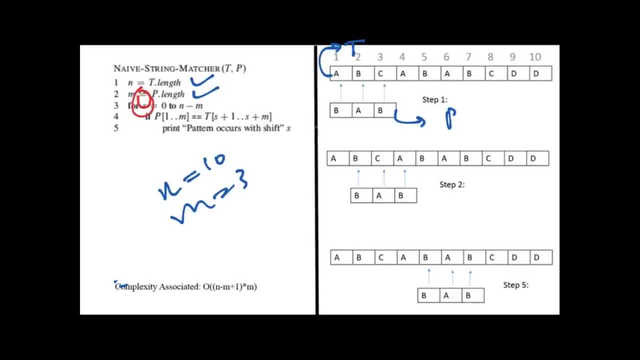 For the matching purpose. there is something very special I need to tell you about. It is s. s is basically the shift. Shift also acts as a flag of telling us if we have found the pattern or not, And shift also acts as a counter. 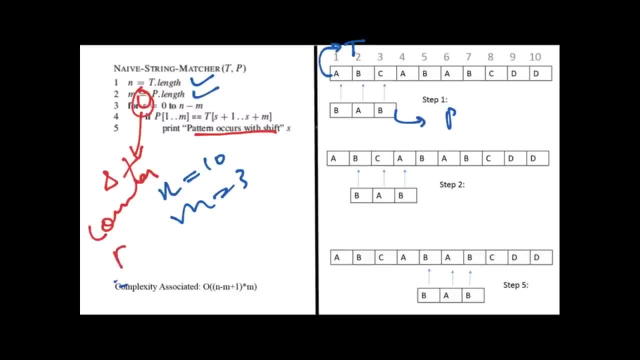 So it does two works Counter. Sorry for the handwriting And the flag. Now we will start matching. Our shift is at 0.. 0. The shift by itself. Actually, the shift is not at 0.. The shift is at 1.. 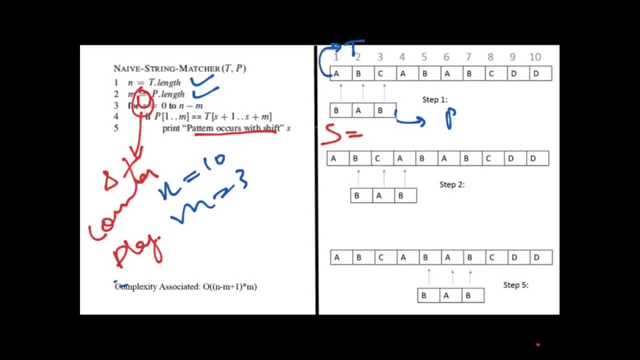 We will start matching. When the shift is at 1, we can see the text contains a, b, c And we will match it with b a b. It is not matching. We will move the pattern one shift ahead. That means now shift is equal to 2.. 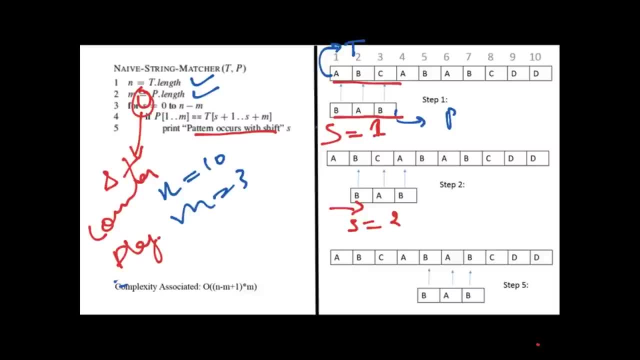 And the previous shift, as you can see, was 1.. Now we will increment the shift to 2.. As you know, I incremented the shift. We will again check if b c a is equal to b a b. We can see that it is not equal. 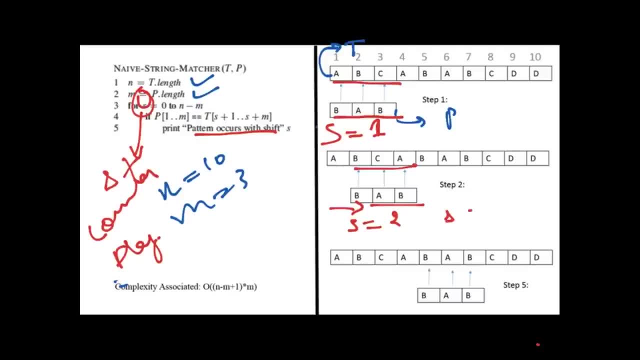 So we will again put the shift to 3.. When we put shift equal to 3, then we can see there is c a b Which is again not matching with b a b. We will again move shift equal to 4.. 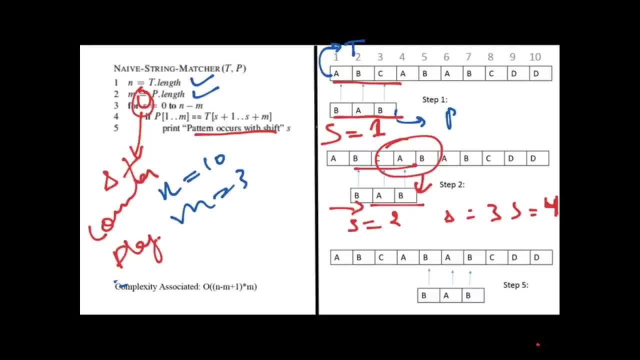 We have moved shift ahead with 1.. And after moving the shift ahead with 1., We can see that it is a, b a, Which is not again matching with the pattern. We will again move the shift to 5.. And here we can see that b a b matches with the text: b a b. 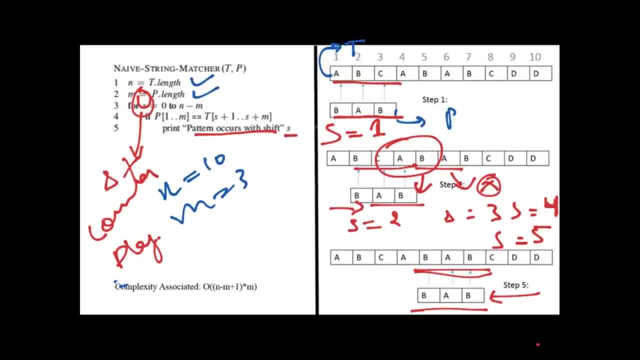 So we can say that the pattern occurs at shift s. We just have to say that at shift s, equal to 5, we have found the pattern. That's all. So you can see, it is the very basic thing. And one more thing I want to tell you. 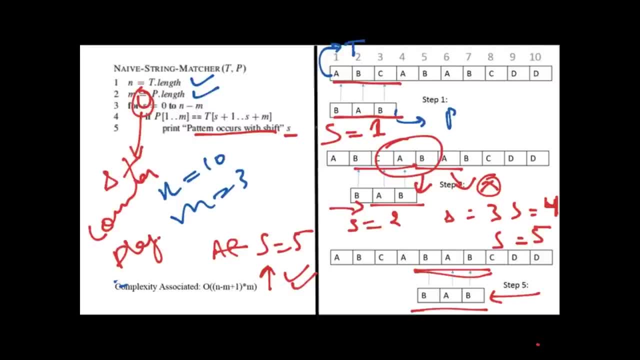 I am just going to correlate the whole algo with this thing. As you can see, the length of the text is 10.. So n will get the value of 10 over here. Then I am talking about m. m will get the value 3.. 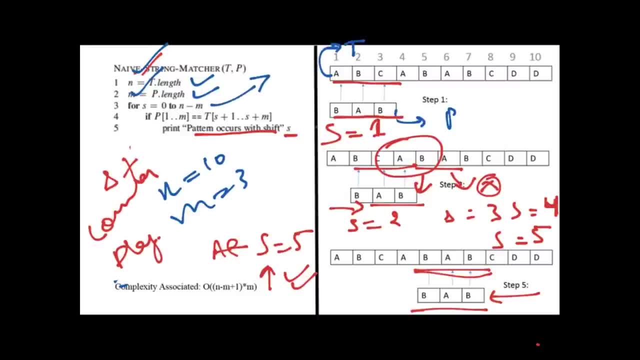 Then, coming to the for loop, As you all know, for loop is used for a repetitive process And we will be basically checking each and every loop With the other letter that is present in the text, as well as the pattern. So we will be checking p 1 to m. 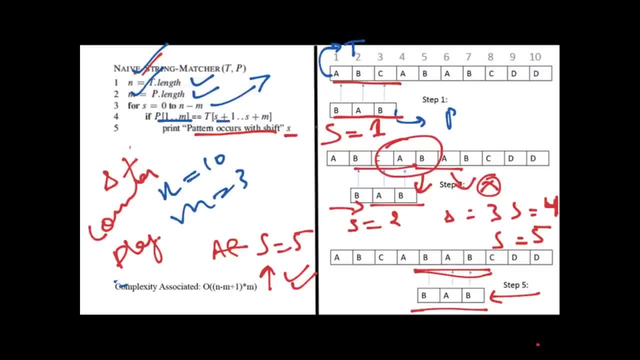 1 to m is basically just for the algorithm, And t s plus 1 to s plus m. Here, s plus 1 signifies that the basic value of s, which was already 0, has been changed to s plus 1.. That means it won't be counting anything from the outside. 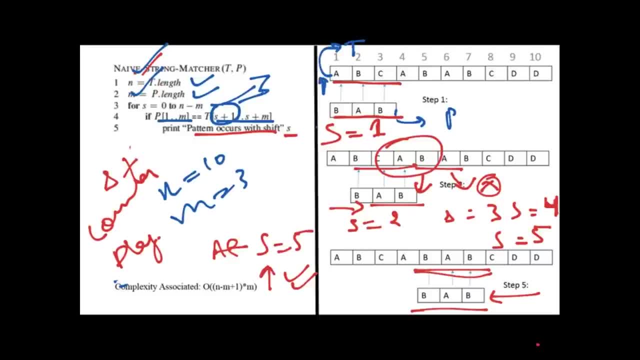 It will be counting everything from the inside. From the inside means from the first position itself. So it will be checking each and every letter, Each and every letter from pattern p and each and every letter from pattern t. This double equal to operator, as you can see over here. 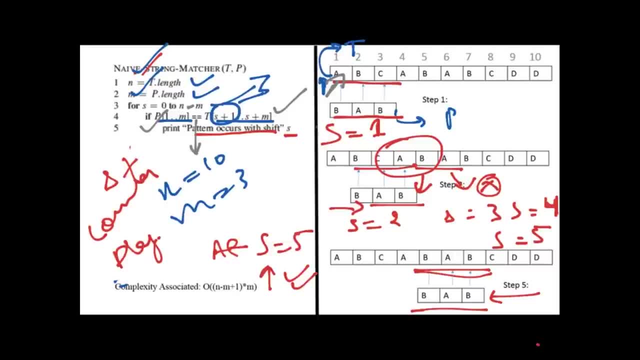 Checks if the value on both sides are equal or not. And as soon as we get that the patterns are equal- Pattern that is present in p and pattern that is present in t- We will assume that pattern has occurred on a shift that is equal to s. 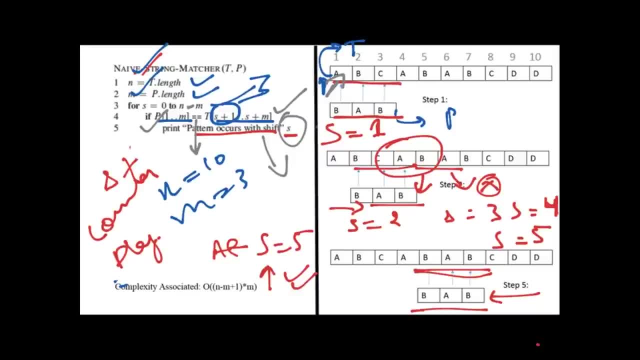 So it was extremely simple. I hope you really liked the video. Thank you so much for your time. Bye, Take care.